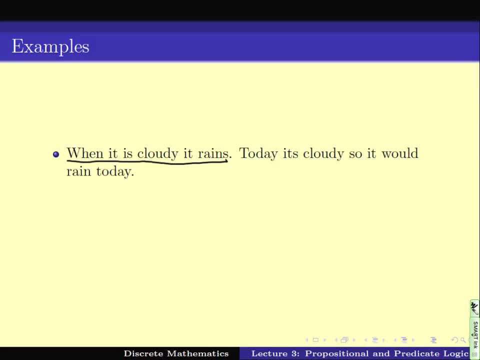 sentence when it is cloudy, it rains and the sentence today it's cloudy are both part of the assumption And what's the deduction? The deduction is it would rain today. As you can see, the assumption comprises of two statements and ideally one should think: 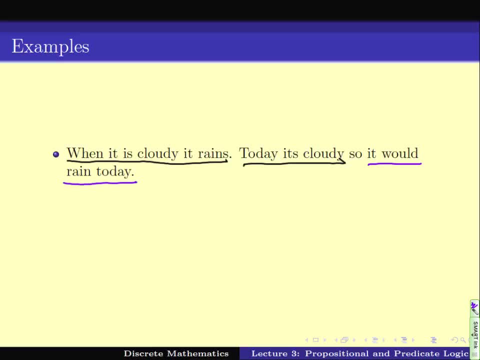 of it as when it is cloudy, it rains, and today it's cloudy. That is the assumption and the deduction is it would rain today. So we see that the assumption is composed of two statements and connected by the connective. AND Now, when it is cloudy, it rains. this can be true or false. 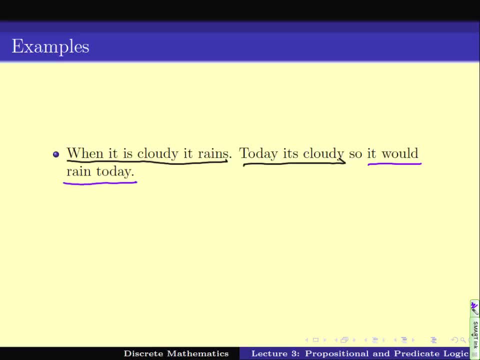 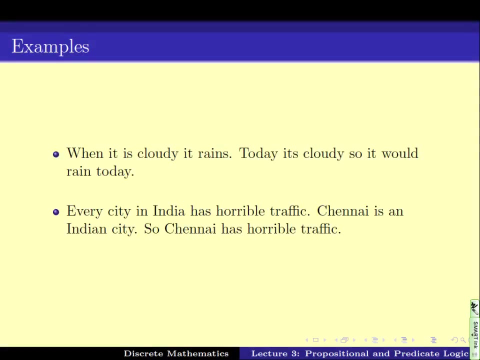 Similarly, today it's cloudy, Can be true or false, So that each of the individual statements can either be true or false. Similarly, consider another example. every city in India has horrible traffic. Chennai is an Indian city, So Chennai has horrible traffic. Now what is the deduction here? 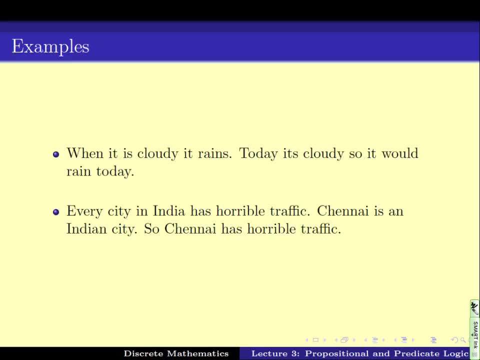 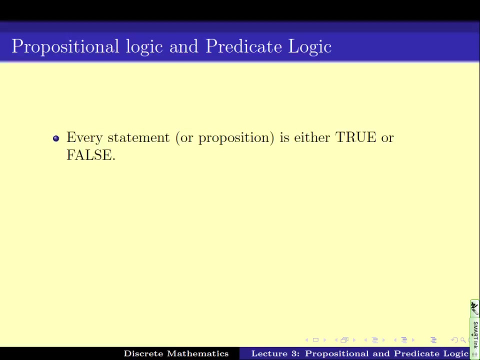 The deduction is: Chennai has horrible traffic. What are the assumptions? What is the assumption? The assumption is: every city in India has horrible traffic and Chennai is an Indian city. So, formally speaking, in propositional logic and predicate logic, we say that every statement. 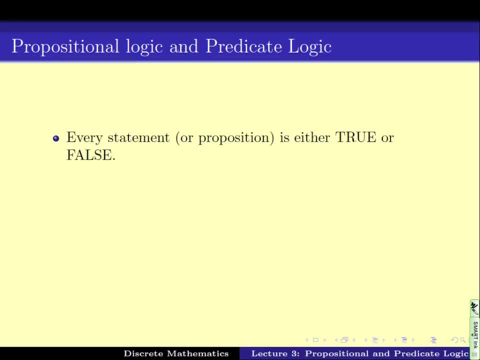 or proposition is either true or false. This is the assumption. This is the assumption. This statement can be composed of other smaller statements and they can be connected using five different kind of connectives. AND OR NOT. IMPLIES AND IF, AND ONLY IF. 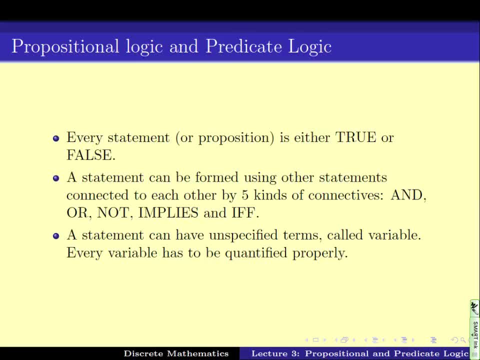 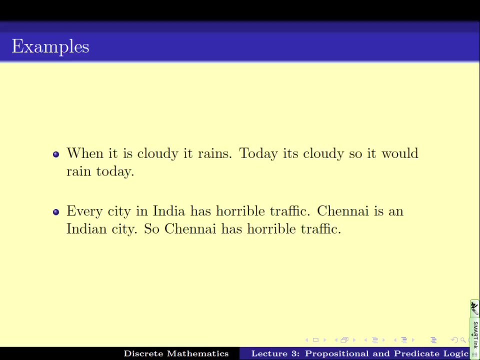 A statement can have unspecified term called variable. each variable has to be quantified properly And this is an assumption. And this is an assumption. Let us go back to the examples that we were seeing just some time ago. So in the first example, as you can see, there are no variables. 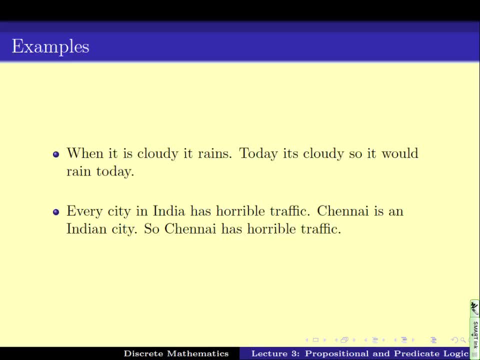 It says that when it's cloudy, it rains. And today it's cloudy implies it would rain today, And when it's cloudy, it would rain. And when it's cloudy, it would rain today, And when it's cloudy, it would rain today. Thus, we had three different statements and they are connected by the connective. 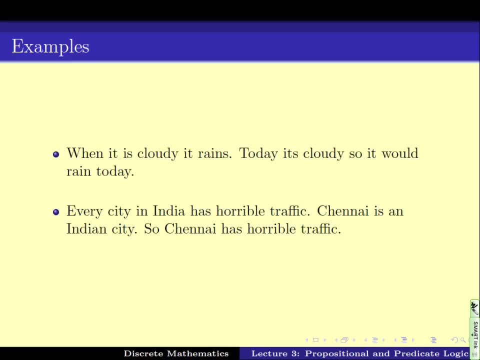 AND and implied. On the other hand, in the second example there is this statement: every city. Now I have not told what city or which city and so on. So this statement every city in India has horrible traffic is a statement where the city is a variable, and this term every city is kind of used to quantify. 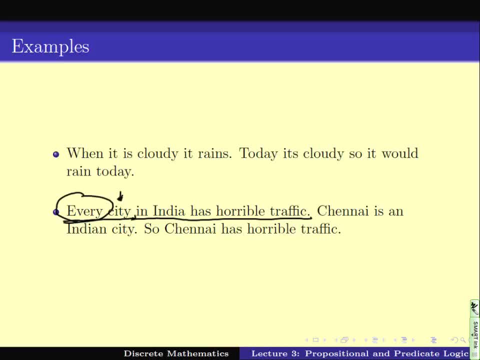 the variables. So we have every city in India has horrible traffic in the statement having a variable which is quantified using this, the quantifier every, And we have the whole sentence as every city in India has horrible traffic. and Chennai is an Indian city implies Chennai has horrible traffic. You. 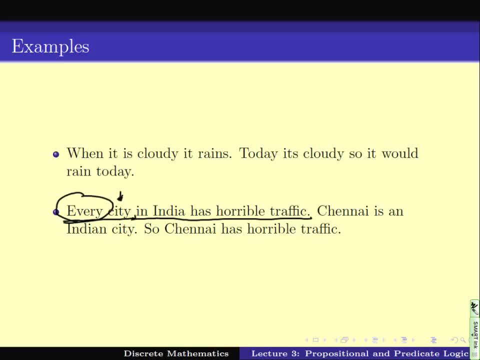 should understand that when we write something in English, we need not use the exactly same words as the connectives, for example, and or implied If and only if and not. We might use something else, some other synonyms. So to understand an English sentence, we have to understand what is the inner meaning. 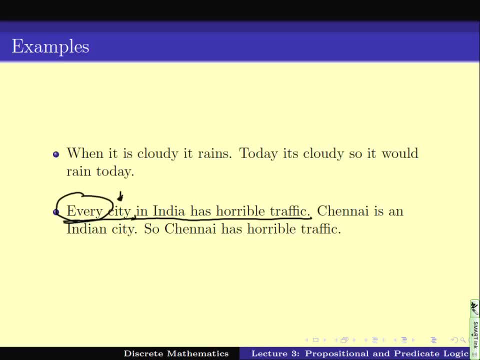 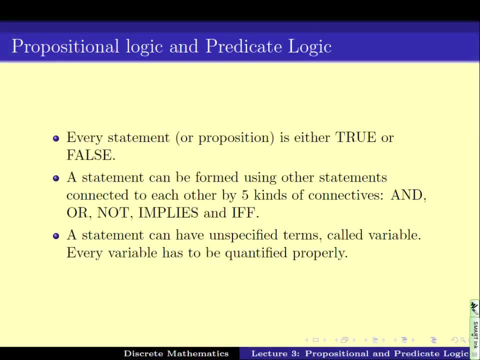 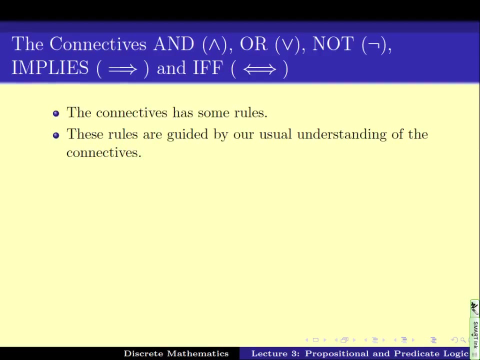 of that, So and that. AND can be replaced by a full stop or something like that. as you can see in this- two examples. Now the connectives of an English sentence are ident. plague phonetically Can be and work Once again. So at the beginning of the sentence we say: 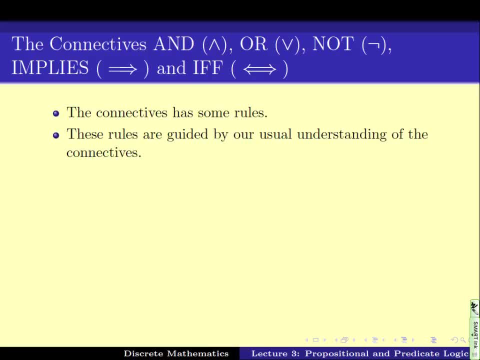 yin and yang. By the way, Let me explain this. so the concept of AND WARいうこと, And says: if I don't live, if an olive fique, some rules, and this rules are guided by our usual understanding of connectives. 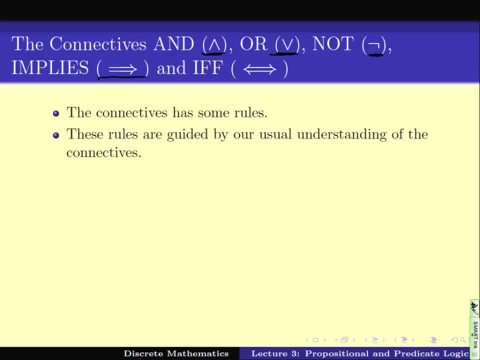 rules are guided by our usual understanding of connectives, by the way the connective and Mathematical is represented using this particular notion: North in the present, within the inverted T, North in this exam. with this notation implies: with this implication, mark an if and only if, sign owl訒 en English. spike an index. 그 prominent или involving any such notation means just a valid reading. the inverse First four words are present and they are all uppercase. if and only five to two, laughing over the to necks while bleeding is triangle, not it is, they are represented étant. 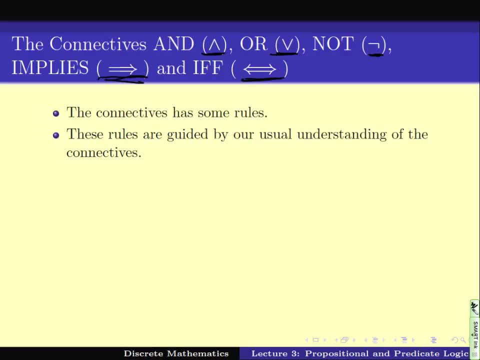 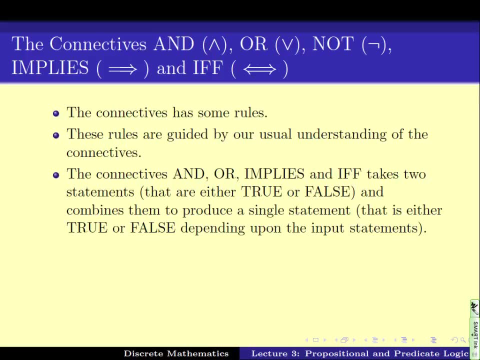 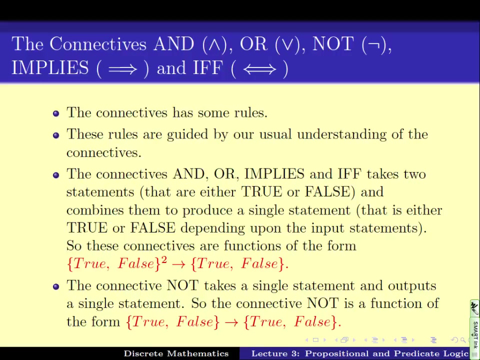 leaf with the double implication mark in either direction. Now the connective and or implies an if and only if. takes two statement, each of which are either true or false, combines them to produce a single statement that is either true or false, depending on the input set. So in other words, these connectives are a. 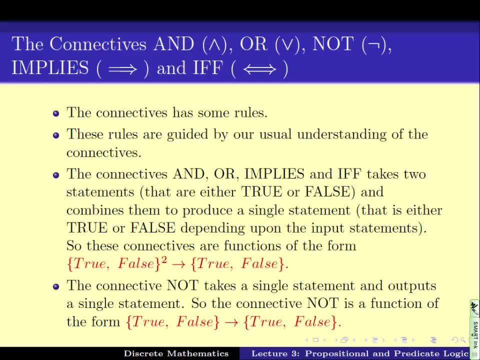 function from true comma false whole square to true comma false Connective. NOT takes a single function and produces a new function. So the NOT is a function from the set true comma false to the function true comma false. Let's see some of the rules that are used for: AND OR IMPLIES and IF and ONLY IF. So here is: 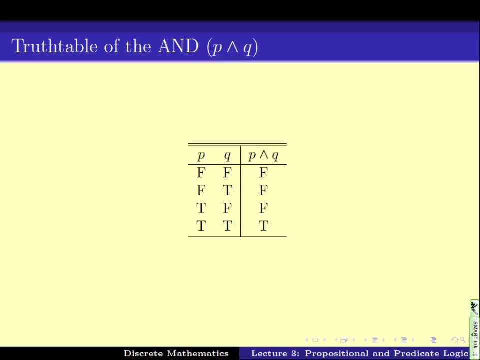 the truth table. You can go over the truth table and you understand what does it mean by each of the statement? Now, this is the way we should read it. So if P and Q are the two statements and we are saying statement like P and Q, so if 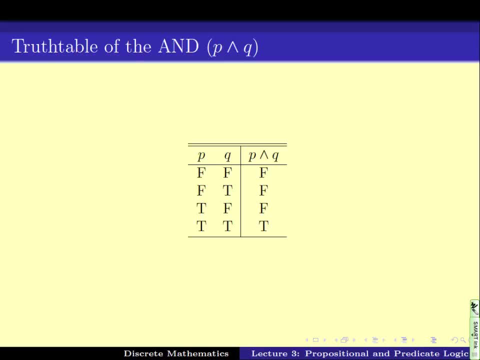 P is false as well as Q is false, then P and Q as a statement is false. This is kind of natural, Like when we say that this happens AND this happens, and if any one of them doesn't happen, it means that the whole thing as a whole also. 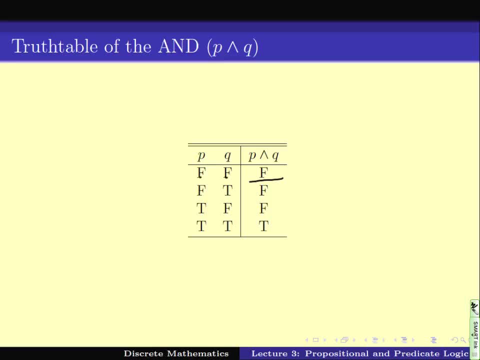 doesn't happen. So false AND false gives false. Similarly, false AND true gives true, True and false gives false. and the last one is: true and true gives true. That means only when both P and Q are both satisfied or they are both true. 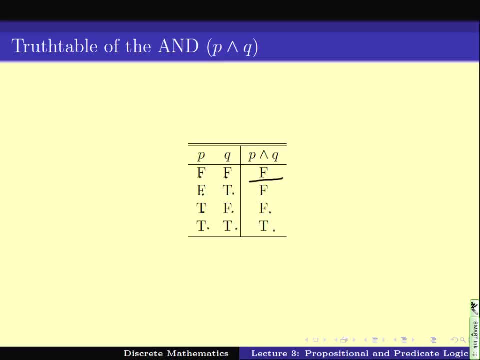 statements, only then the combined function of P and Q is also true. Similarly for, or. for example say: if I say that I will either give you an A grade or I will give you an B grade, Now this says that as long as I do either of 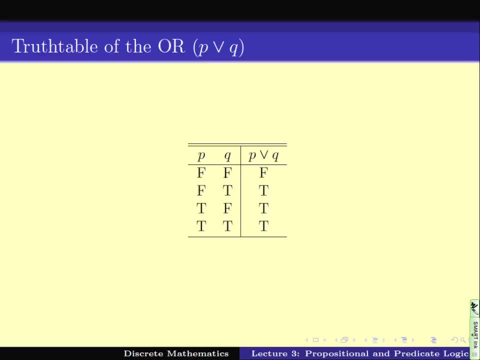 those two objects, the whole sentence is true. So in other words, as long as one of P and Q is true, I get true, Whereas if both of them are false, then the function evaluates to false For the connective. not, it just flips the function, It just adds a negation to the statement. and 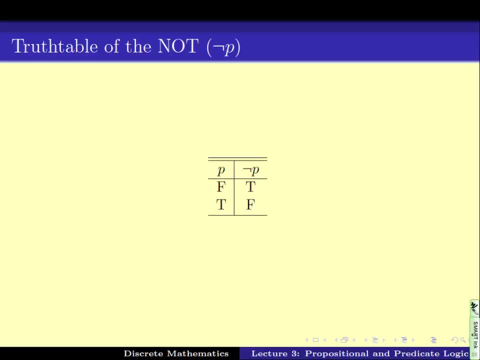 just a false statement becomes a true statement and that true statement becomes a false statement. Now let's consider this interesting function of implies. When can you say P implies Q is a right statement? So when the mathematicians and the logicians were setting up the mathematical foundations, they were divided as to how to define. 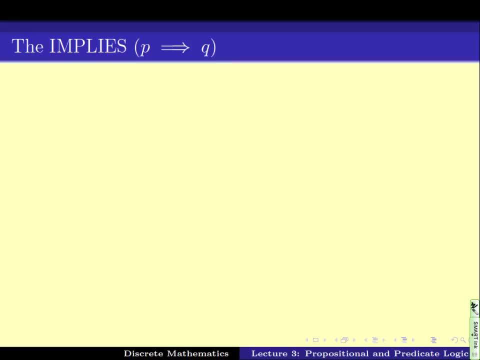 this particular function implies. So one thing that they decided is that a true statement always proves the true statement. Hence, if P is true and Q is true, then the function P implies Q is also a true statement. At the same time, P cannot imply the false statement. 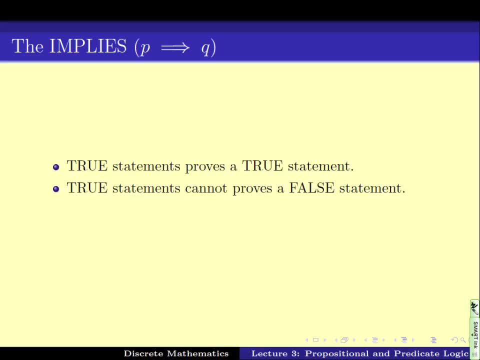 That's the other way of saying. So if p is true and Q is false, then the whole statement has to prove to be evaluated to false. Here is one slightly more complicated thing: that a false statement can prove any statement. So in other words, if P is a false, 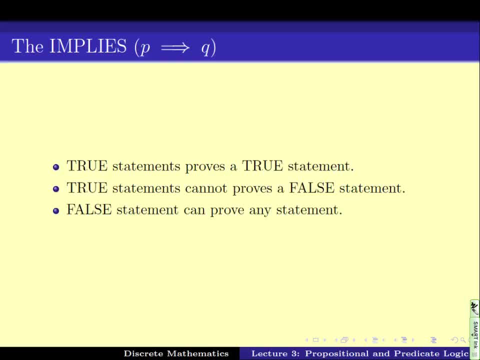 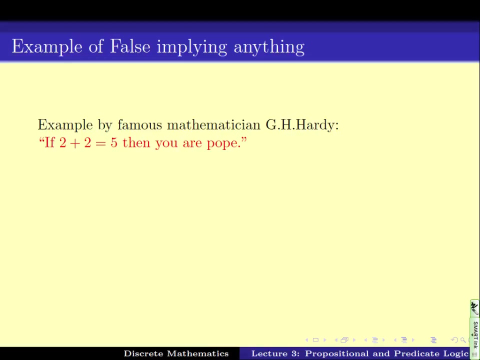 statement. from that I can imply anything. which means false implies true is also true, as well as false implies false is also false. There was lot of debate on this, and one example of one beautiful story that goes along is that when the mathematician GH Hardy was asked to comment on this statement or was asked to 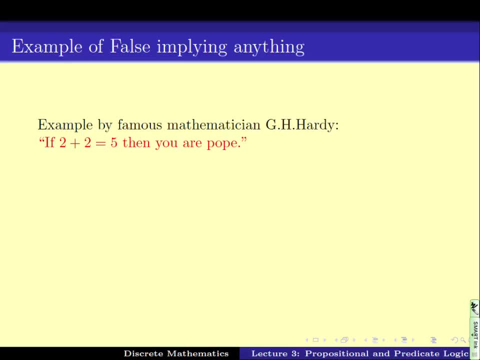 comment on this particular rule, for implies. he was asked to prove that. can you prove the following statement: if 2 plus 2 equals to 5, then you are pro. Now, clearly, 2 plus 2 equals to 5 is false and you are. pop is also false. 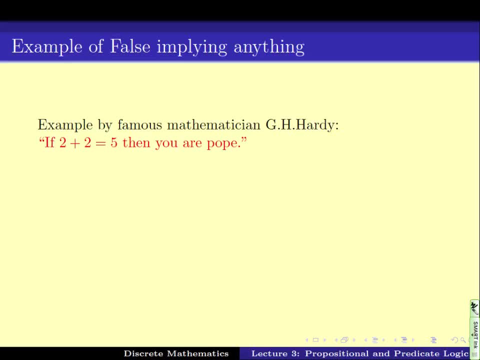 statement. Now can the false statement imply any false statement. for example here- and GH Hardy did give a proof and here is a very cute proof of that- It says that 2 plus 2 equals to 5. now, everybody knows: 2 plus 2 equals to 4. 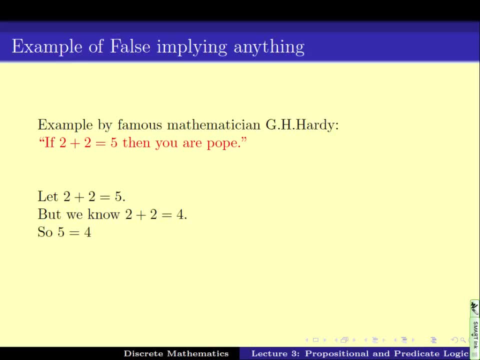 that means 5 equals to 4. if we subtract 3 from both sides, you get 2 equals to 1, so 2% equals to 1%. therefore, you and pop are 1%, hence you are pop. This is a very cute proof or very cute example that shows. 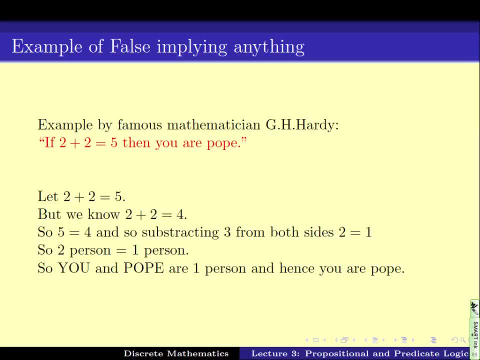 that if you assume something is false- in this case, 2 plus 2 equals to 5- then you can prove any ridiculous statement or not. for example, you are pop. So in other words, for the case of implies, it is accepted that a false statement implies any. 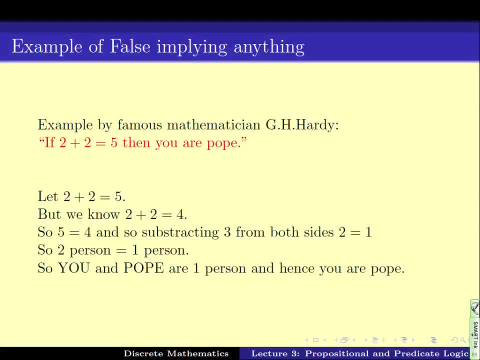 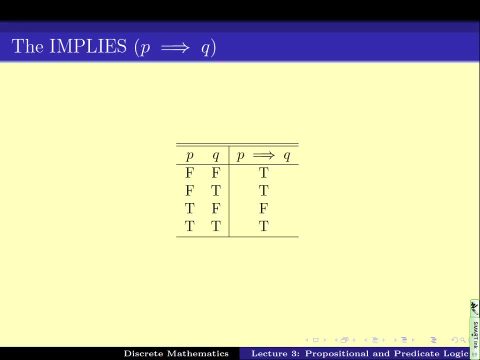 statement. Thus, the truth table of the implies function has false implies false is true, false implies true is true, true implies false is false and true implies true is true. Similarly, we have the other thing of if and only if, and I leave you guys to convince yourselves that this particular truth table also makes sense. Now there 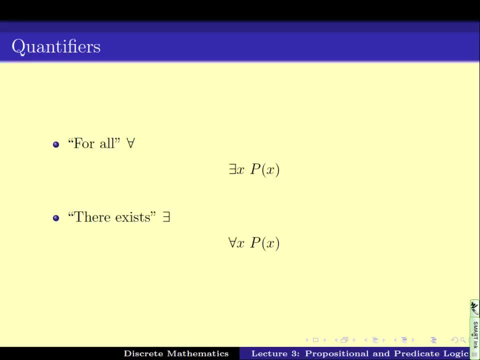 are two quantifiers also that are there. as I told you, every variable has to be quantified and these quantifiers are for all and there exist, And you write step-by-step like this: So this says that there exists X, such that P is true. This is. 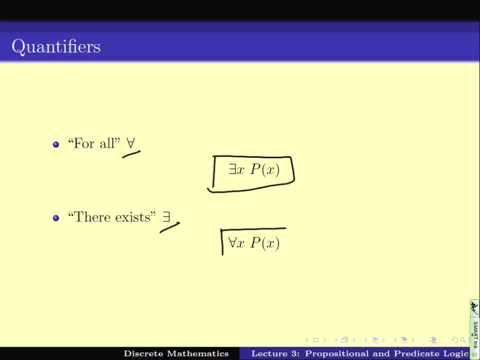 how you should read the statement. Similarly, this one says that for all X, the statement P is true. If you recall the example we had used, there was this example of every city in India has horrible traffic. So in that respect, X is the city. every means for all, So for all city, and the statement was the city. 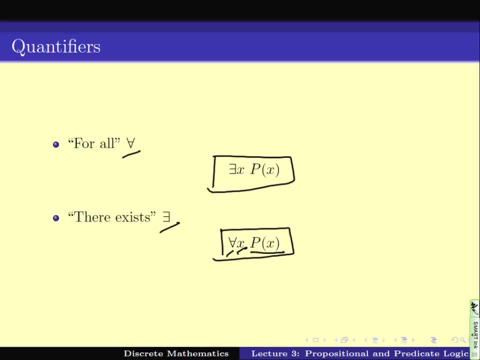 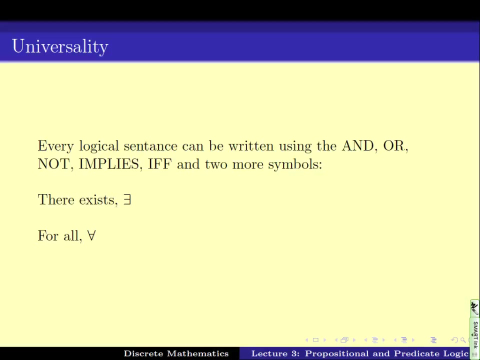 has horrible traffic. So it should read: as for all city in India has horrible traffic. Now it's a nice, important fact that using these five connectives and the two quantifiers there exist, and for all, one can write any logical statement. So these: 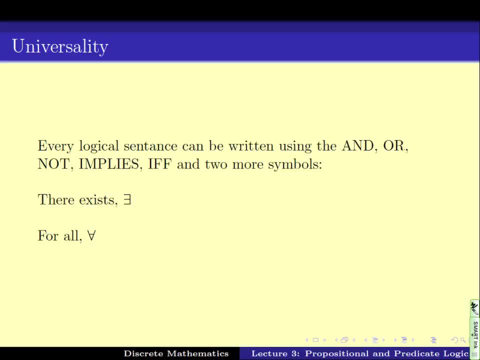 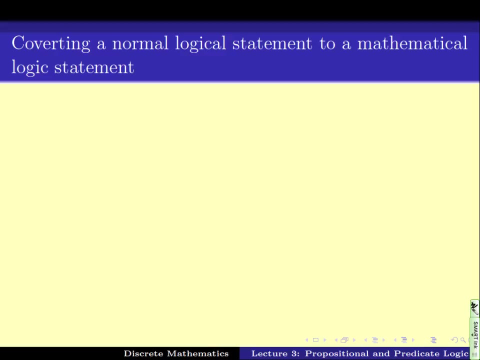 are called kind of universal set of notations using which any logical statement can be solved or written. Let's see some example. Let us take a normal logical statement. to a mathematical logical statement, For example. consider this particular para. This says that if you did not know the material earlier and you don't study, 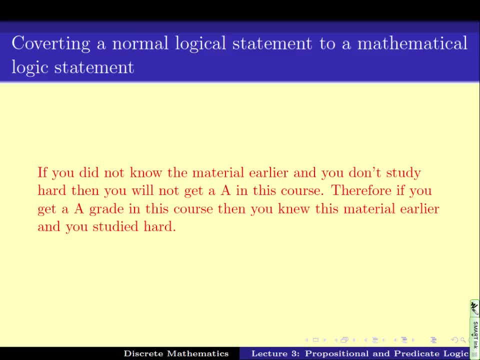 hard, then you get, then you will not get a A in this course. Therefore, if you get an A in this course, then you knew this material earlier or you studied hard. Now I would like to check the logical validity of the statement. First of all, we should: 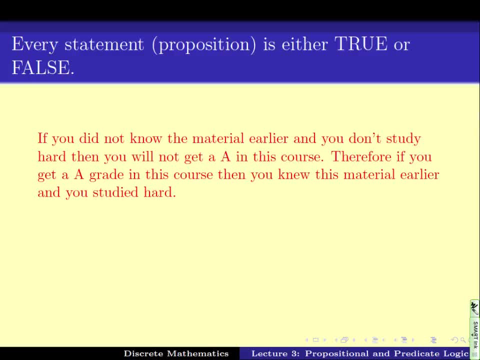 understand that this statement as a whole is either true or false. And if this statement is true or the statement is valid, if, for any condition satisfying the premise or assumptions, the statement holds true. So in this particular case, you have to understand what are the premises, what are the deductions. 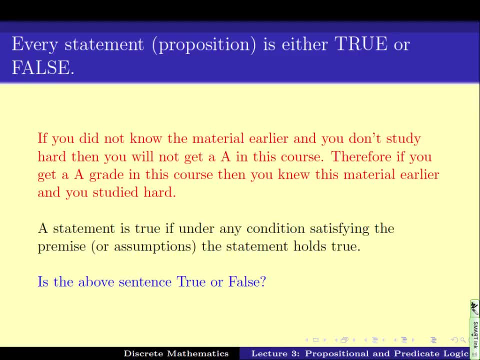 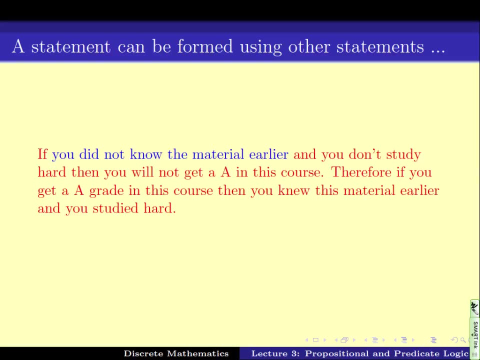 and what are the connectors? So if you want to ask, is the above statement true or false, let's try to convert it to a mathematical statement To start it. as you have seen, a statement can be formed using other statements, For example here. you did not know the material earlier. 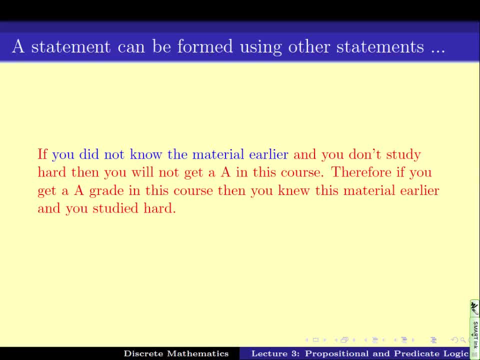 Either smaller statement. This statement can either be used, Either be true or false. Either you knew the material earlier or you did not know the material earlier. In any case, this is a statement that can be true or false. Similarly, you don't study hard the statement that can be true or false. 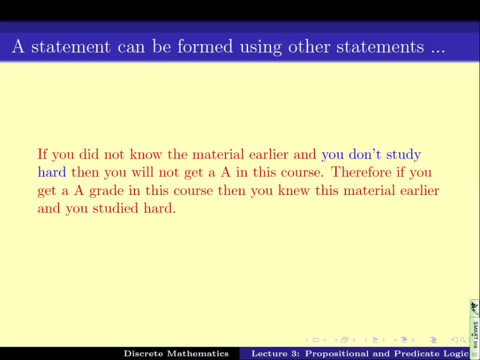 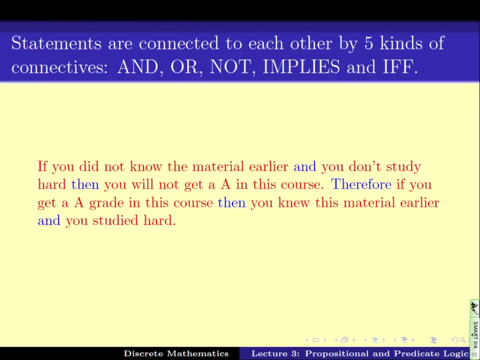 There are other statements here. I let you guys to look around inside the para and identify the set of statements. So Now these statements are connected using connectives like and or not implies and if, and only if, As I told you earlier, not necessarily this exact set of words of and or not implies, if. 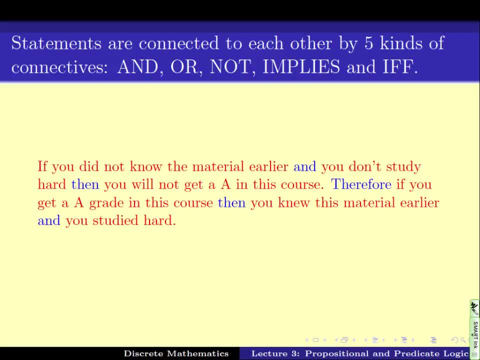 and only if will be used. One can use other synonyms of it, For example, in this case, and then therefore has been used, And then therefore has been used, And then therefore has been used, And then therefore, So then and therefore, are actually synonyms of implies. 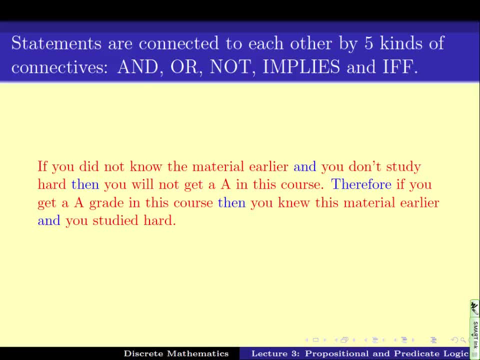 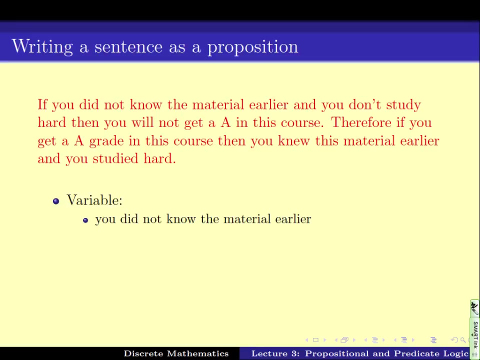 Now, now that we have understood what are the connectives and possibly, what are the statements, let us try to convert this statement or this para, this English para, into a mathematical, the logic, mathematical, logic statement. To start with, Let us start take the first statement that is there, and that is: you did not know the 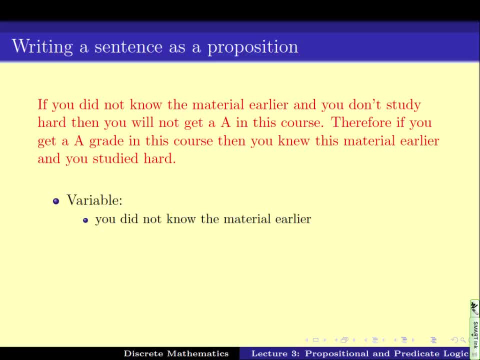 material earlier Now. this is a statement. I don't know how to break the statement into smaller statements, and hence I call this one a variable. Let's call this p. What is the next statement? that is there, It is. you don't study hard. 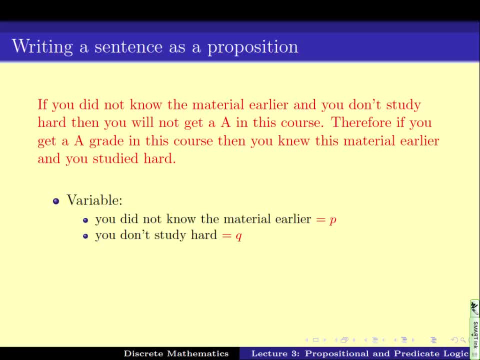 Let's call this variable p, Q. What is the third one? Third one is: you will not get an A in this course. Let's call this one a new variable: R. Now what is the next one? Here is another statement. 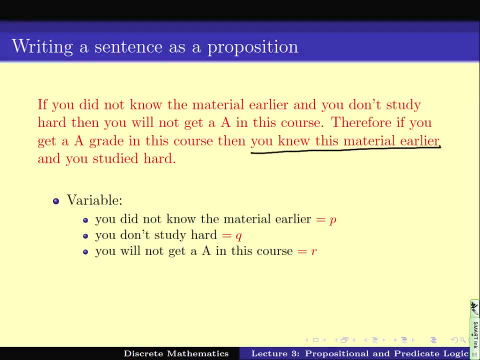 You knew this material earlier. Now, what is this statement? So what is the statement? You knew this material earlier. Note that if p indicates the variable, is the variable indicating you did not know the material earlier, then you knew this material earlier is nothing but not of p. 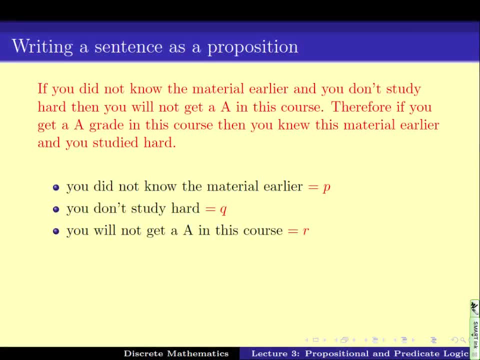 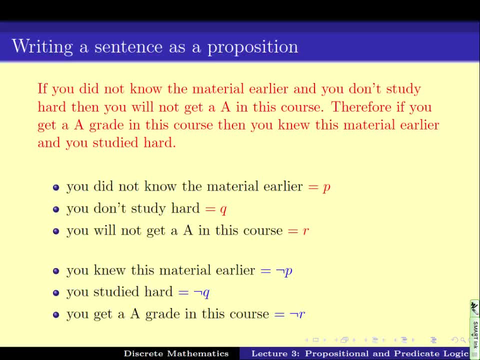 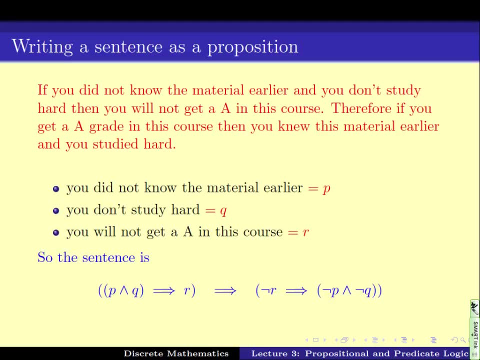 Now, using this set of variables, what can we, how can we represent this statement? Let's see, Let's see, You can check for yourself- that we can write it in this following fashion. And the reason we can write it in the following fashion is that we can read this sentence: 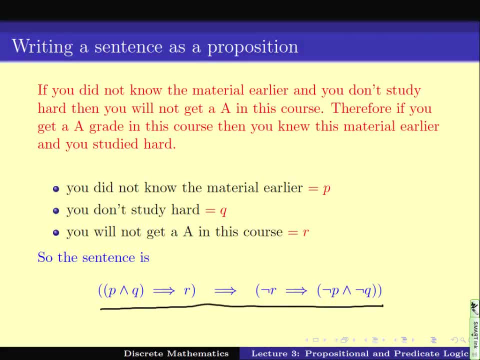 from left to right and you will see that this para coming up completely, For example, since p is- you did not know the material earlier, and so on. I will just replace the p, q and R with the English sentence. So I will just replace the p, q and R with the English sentence. 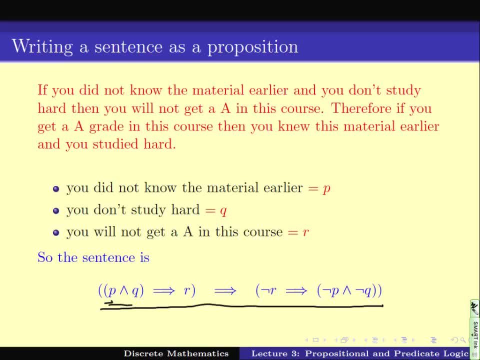 You did not know the material earlier and you don't study hard implies you will not get an A in this course. Thus, or therefore, you get an A in this course implies you knew the material earlier and you studied hard. So this English sentence has been converted into a mathematical logic statement, a mathematical 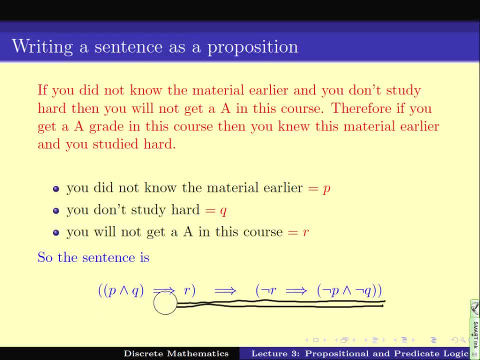 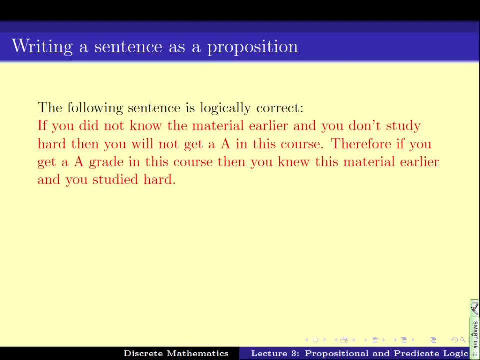 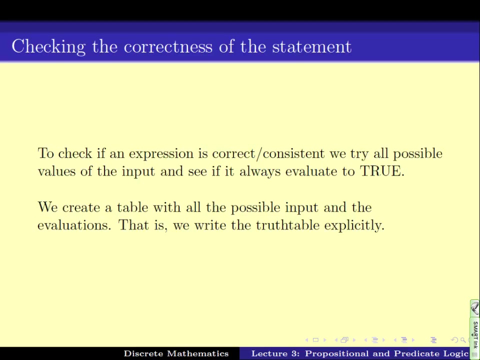 logic statement. Thus the sentence is logically correct. if, in whatever ways, I put p, q and R as true, false, true or false, This following equation or statement must evaluate to true. So to check if an expression is correct or inconsistent, we will try all possible values. 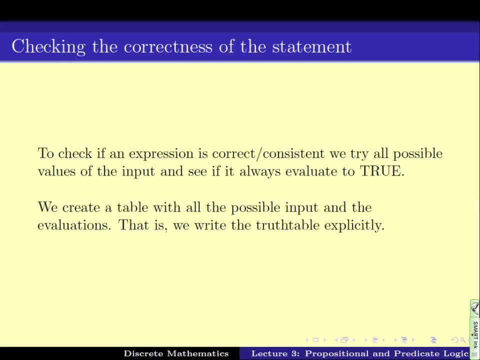 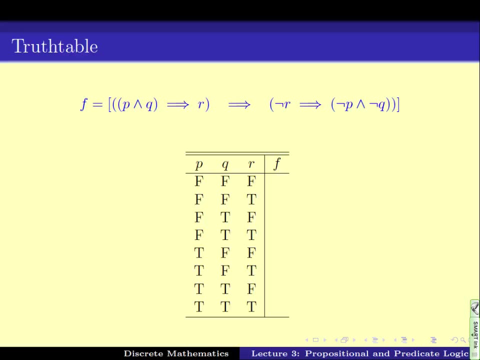 of the input And see if it is, if it always evaluates to true. One way of doing it is to write down the truth table of the equation exactly. That means for all the possible choices of p, q and R set to true and false. 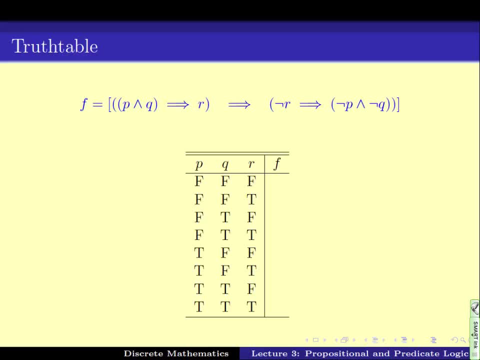 So there are eight of them- Does the function f, which is this function on top, evaluate to true? And the way to do it is to do the whole truth table. Now, as you can see that the evaluating the truth table is a slightly tedious job and 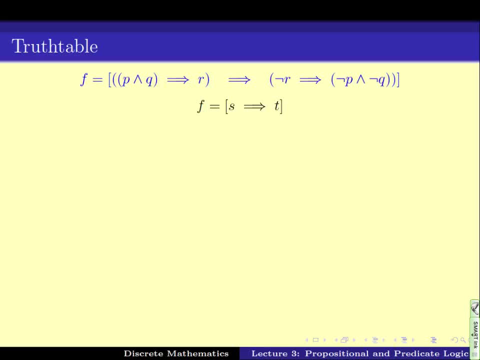 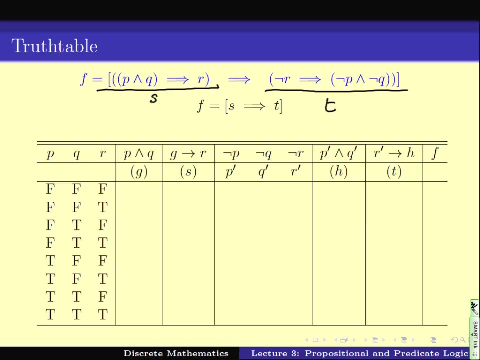 we break it down to smaller parts. Namely, let's say, f is s implies t. That means this is s and this is t. Now to evaluate s I have to write, I have to have p, and q implies R. 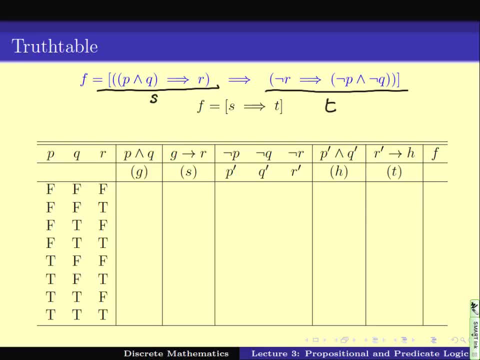 So I first have to evaluate what is p and q, and then I have to go for. p and q implies R, So here is the first few steps. So p and q is following the truth. table of and, And. So that means if both of them are false, it is false. 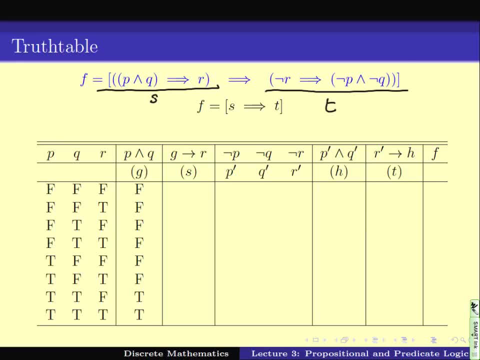 If one of them is false, it is also false, And only when both p and q are true, it evaluates to true. Now, if this is g, g implies R. When is that true? Now, for example, say false implies false is true because, as we have discussed, false. 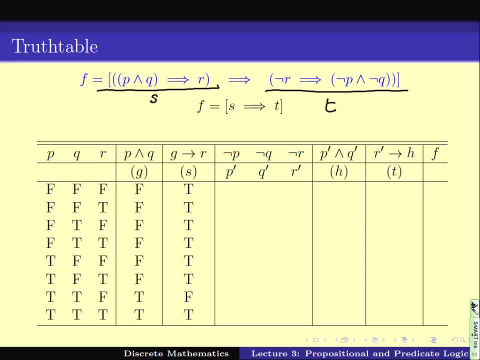 statement implies any statement, So similarly you can do it for all of them. False implies true is true, False implies false is true, and so on and so forth. True implies true is true, True implies false is false, and so on. 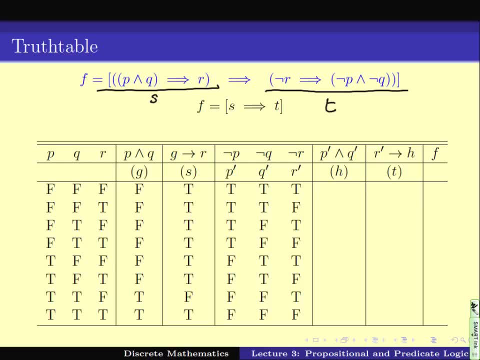 Similarly, we can do the not of p and not of q and not of R, which is using the truth table of not, And then I can evaluate what the value of t is By doing the same thing, First of all doing it as not of p and not of q. 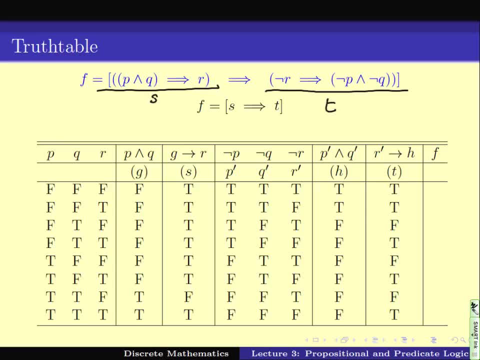 And then not of R implies not of p and not of q. And once we have that, we have this s and we have this t And that s implies t. Let's see: true implies true right, True implies true correct. 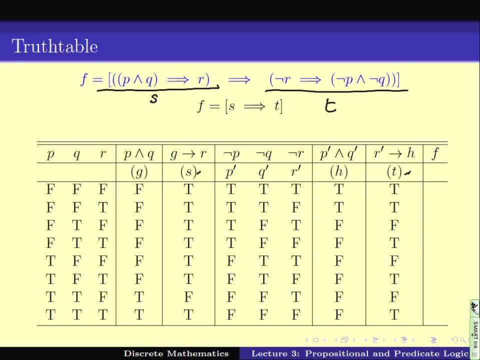 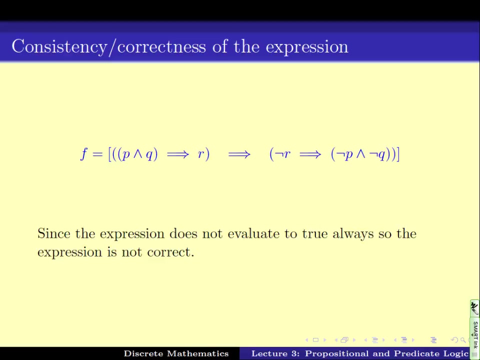 True implies false, And that is not true, That is false. So in fact, when you write down this whole equation, you realize that the function f evaluates to false at two cases and true in the rest. So since the expression does not evaluate to true always, so the expression is not correct. 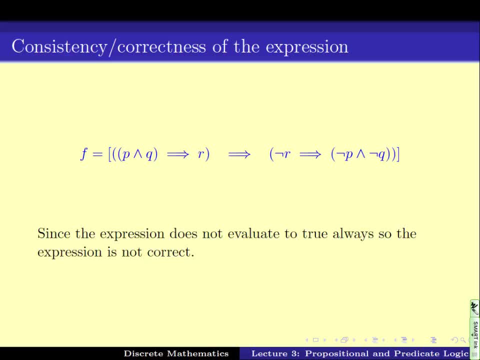 This is possibly something that you could have understood by looking at this sentence as an English sentence earlier also, But here is a mathematical way of proving that this English sentence is wrong. So, to recollect what we have done till now, we have set up the basic for the propositional.